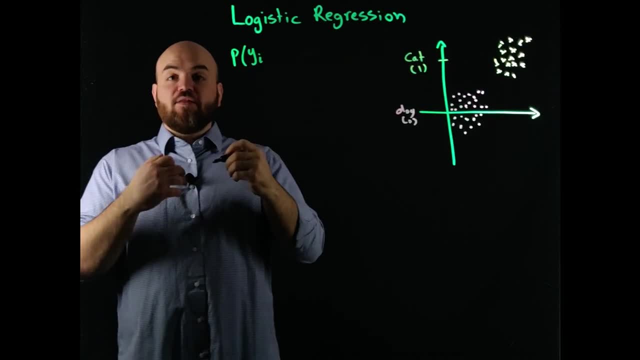 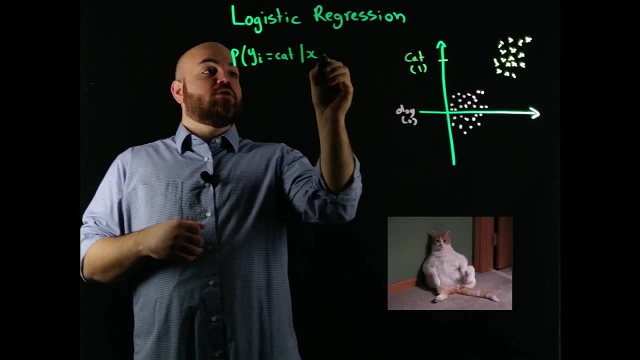 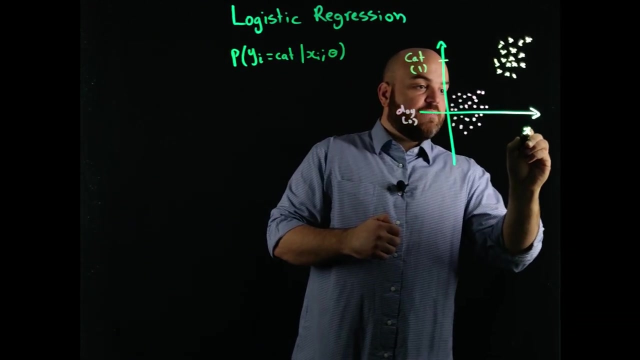 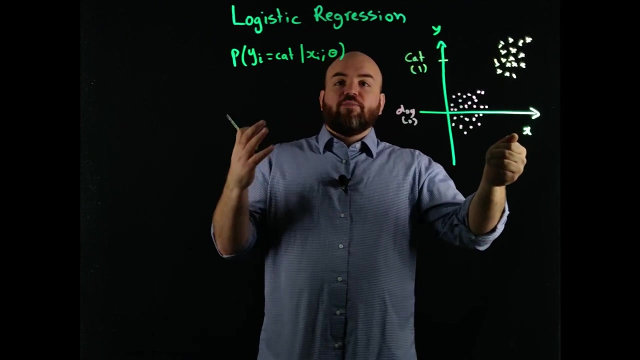 that a dependent variable is of a certain category, say cat, given an input and a certain model. So say I have a bunch of inputs, say these are the independent variables x and the dependent variable y. And let's say these are images. Now I'm displaying those in 2D as one data point. 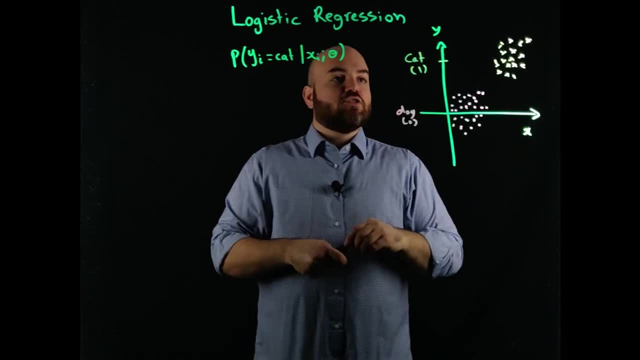 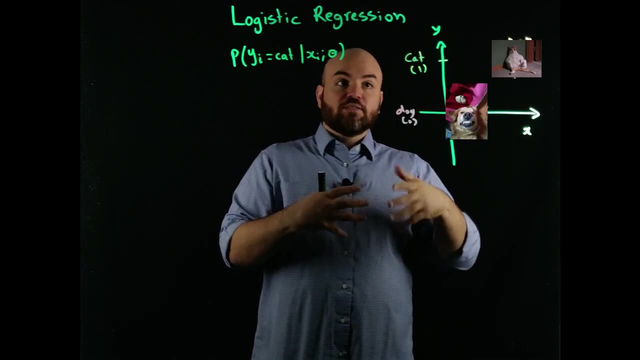 just in order to make the, to make the case for what is logistic regression. But let's just say: this is an image and this image is clearly an image of a cat or clearly an image of a dog. These are categories, so 0 and 1, right. 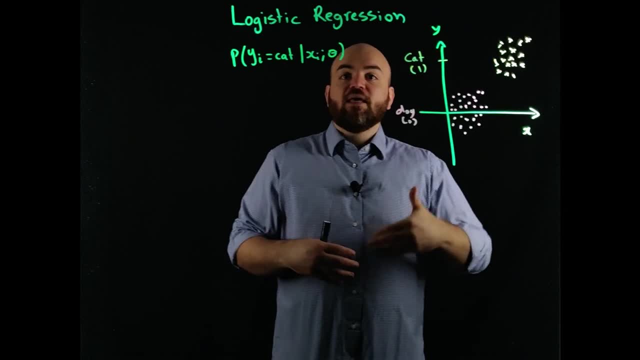 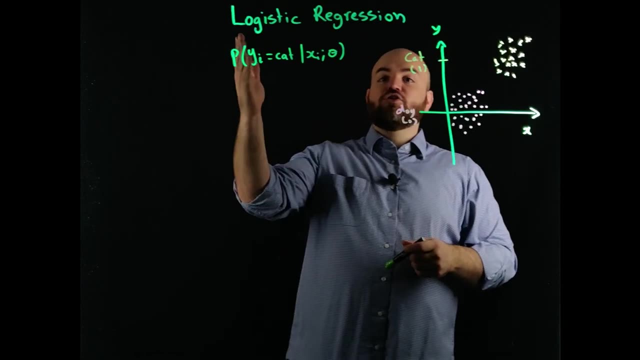 So this becomes a classification problem, And a classification problem is the ability to predict a certain input having the certain type or certain class, And that's what logistic regression does. for us. It's a classification algorithm to find the probability that I've given this input. 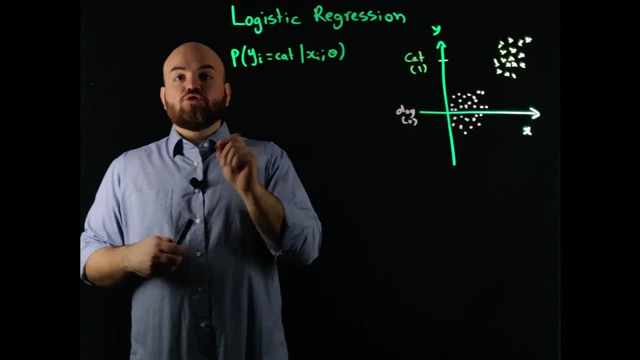 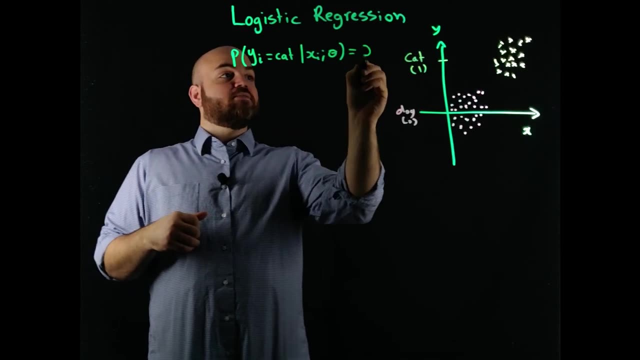 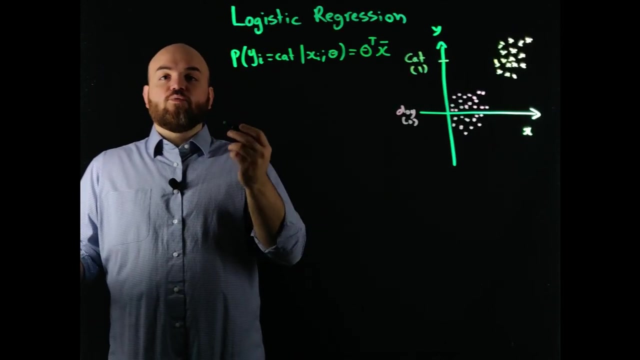 and I have a certain model That that input belongs to a certain category. So how do I do that? Now I could say that I want to use a hypothesis similar to linear regression, right Where I have theta, transpose and x-bar. You can go back and watch my video on linear regression and see what that means. 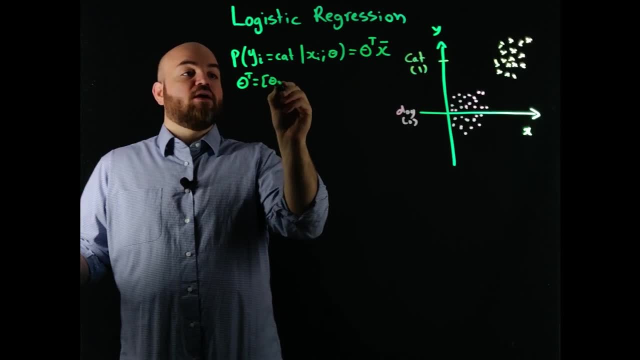 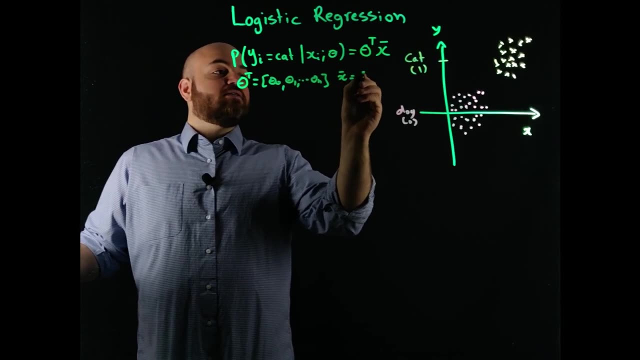 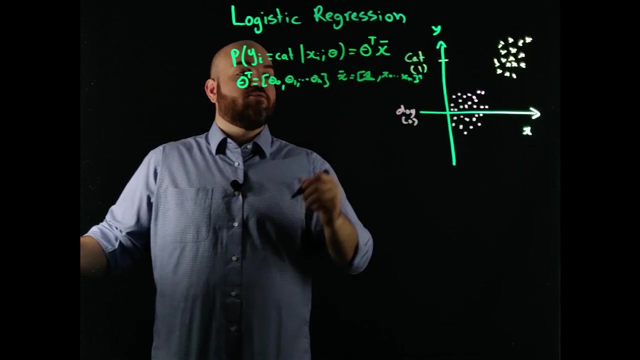 Where I have theta transpose is the row vector of theta 0, theta 1, all the way to theta n, And x-bar is is at 1,, starts with 1, and then goes to x0 all the way to xn. transpose column vector right. 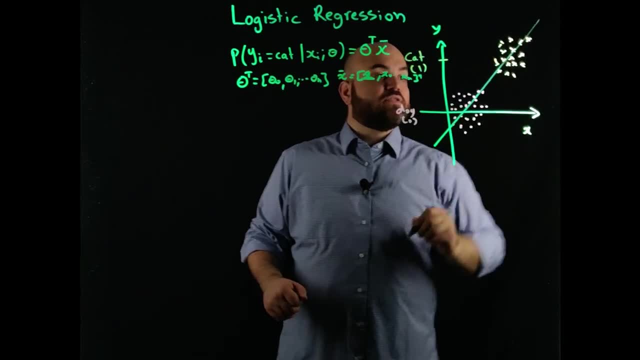 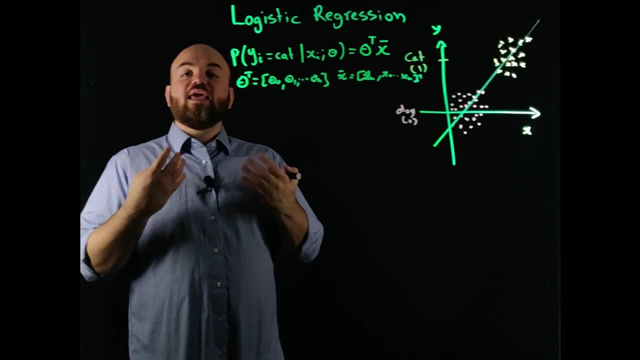 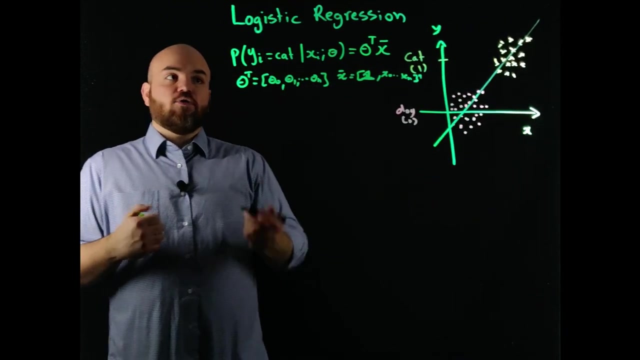 So if I do that, I could then fit this data with something that looks like this: right, But if I want to find the probability of this value, then it can't be that I use a line, because this line can have a value larger than 1 and less than 0, and that violates the definition of a probability. 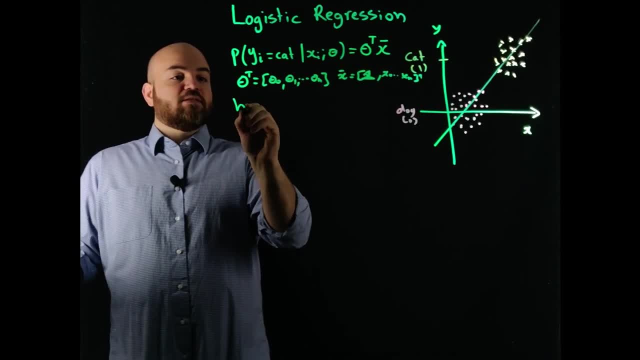 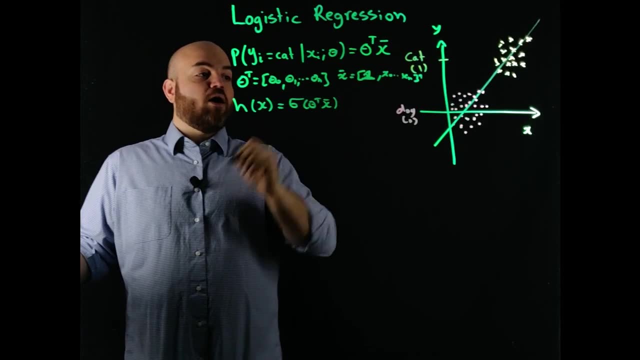 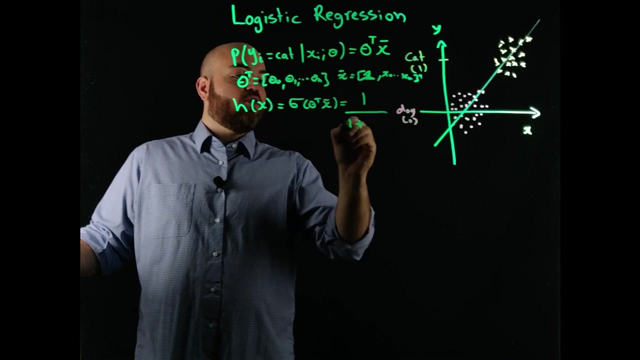 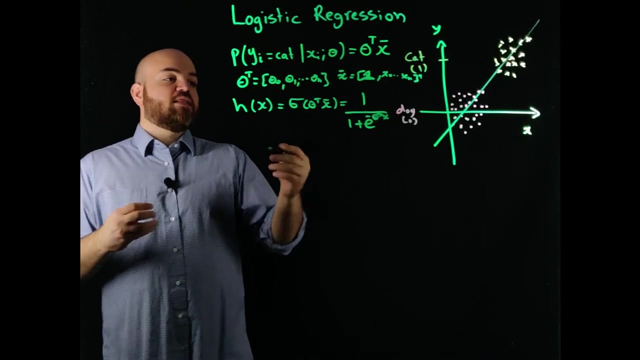 So what do I do? I make my hypothesis h of x equal to some function, sigma of theta transpose x bar. and that function that I pick here is a sigmoid function which is equal to 1 over 1 plus e, to the negative minus theta transpose x. And the reason why I pick the sigmoid is twofold: The 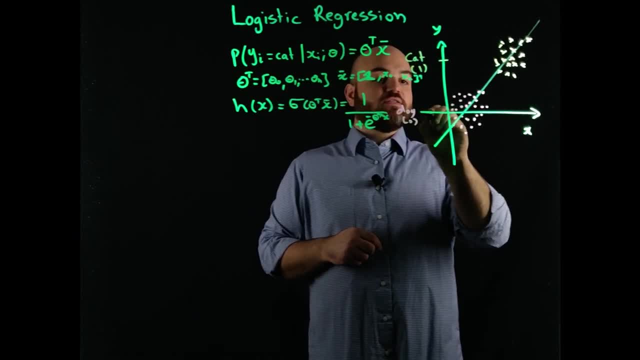 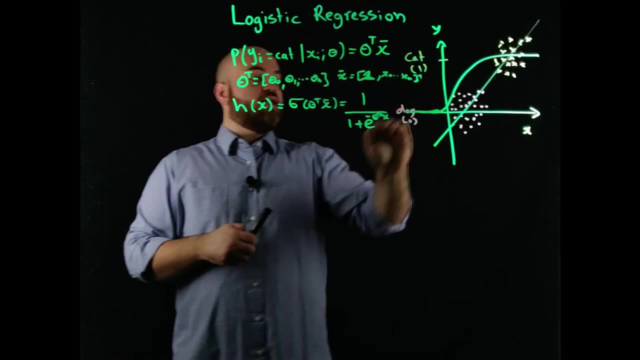 first is that the sigmoid looks something like v. It starts at 0, then it ramps up to 1, right, That's what a sigmoid looks like. So it's squashed here and here. Now technically it goes around 0, so like the 0 axis would be here. but the idea 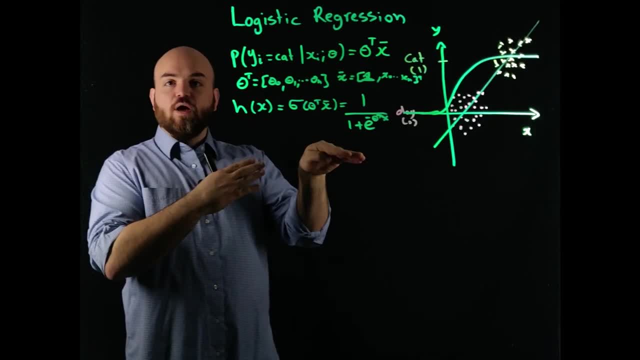 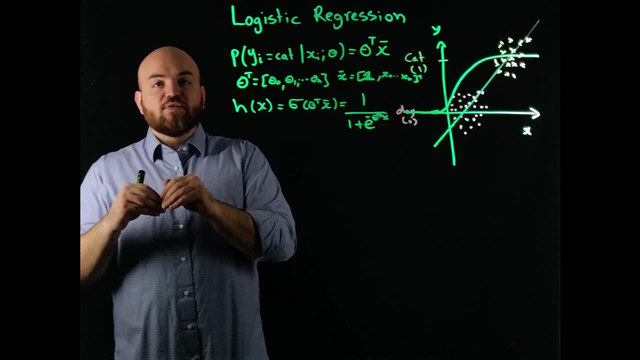 here being is that the sigmoid function cannot be larger than 1,, no matter what the input is, or less than 0. So that's the first reason. The second reason is that the derivative of a sigmoid is mathematically convenient, and we'll find that out later. in general, 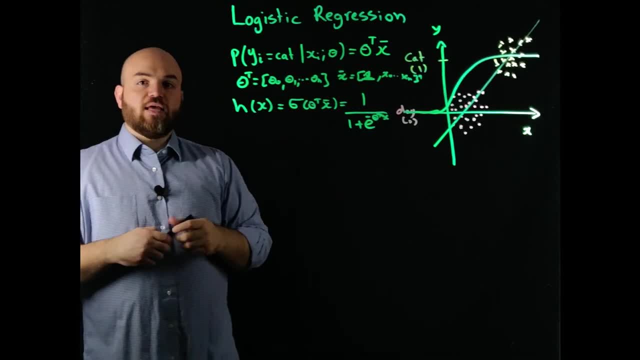 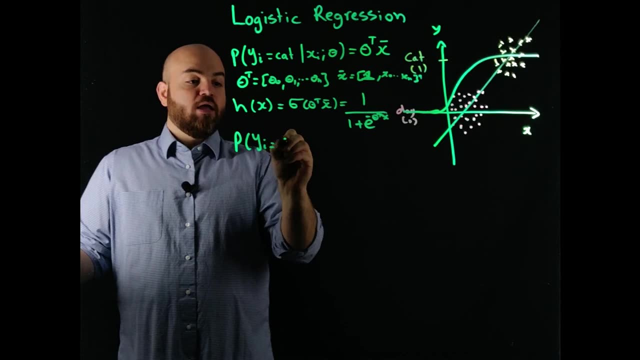 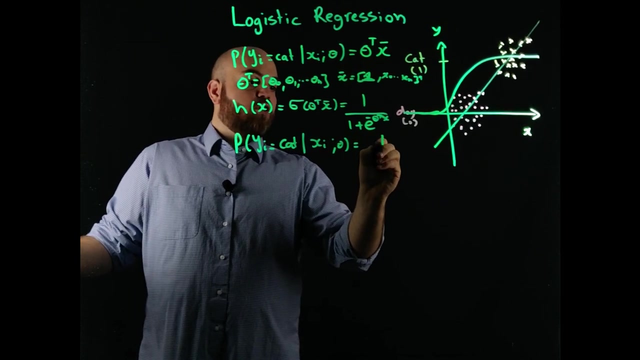 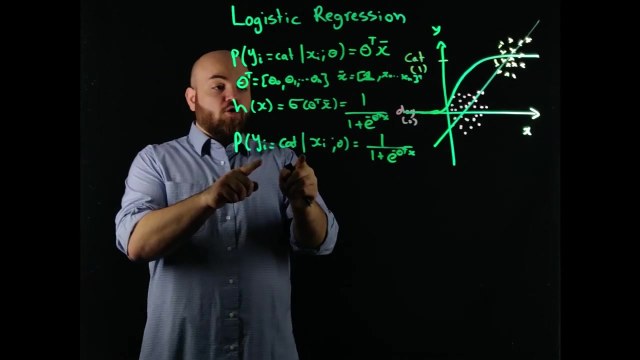 Just a few minutes. However, here that's my hypothesis right. This is the hypothesis that I can find. the probability of yi one sample is equal to cat. given xi parameterized by theta is equal to 1 over 1 plus e to the minus, theta transpose x right. So the reason why the notation 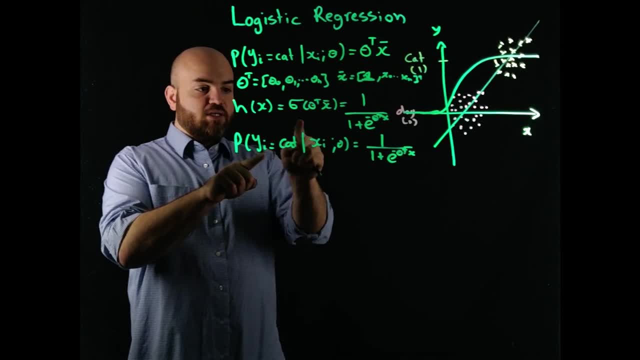 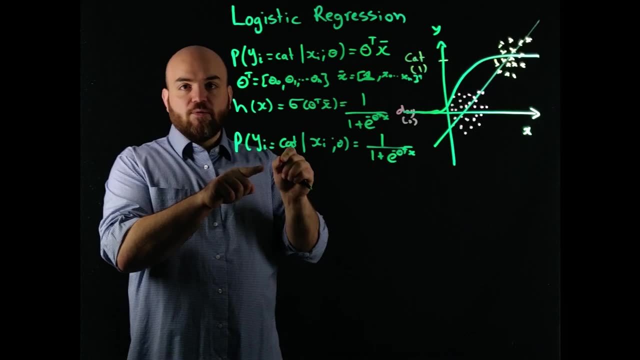 I'm using here is that the probability of y condition so given by this bar means given xi, and I'm putting this semicolon here because theta is not really a random variable. Theta is a parameter that we need to find And also my probability. 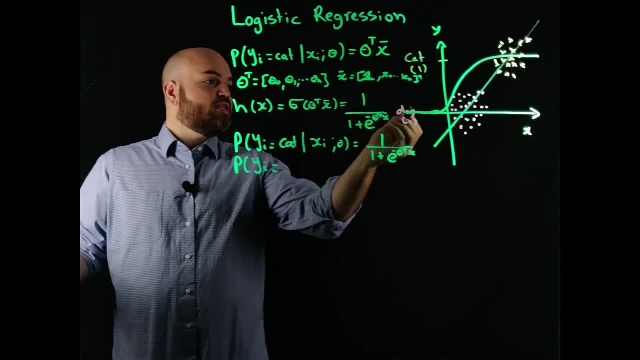 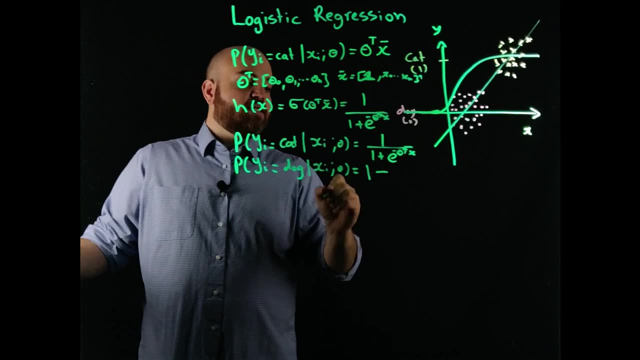 that yi is not a cat or in this case it's a dog. given xi parameterized by theta is going to be 1 minus this probability, So 1 minus h of theta of x. right Now I don't want to say theta transpose. 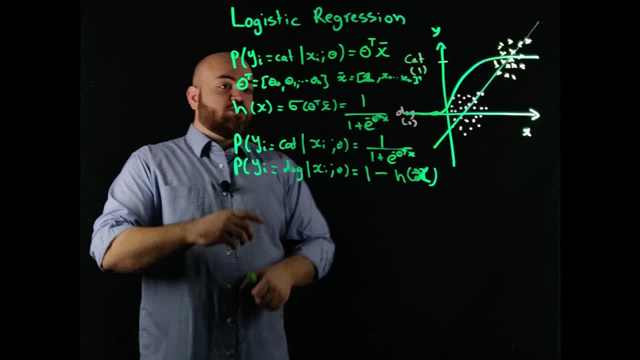 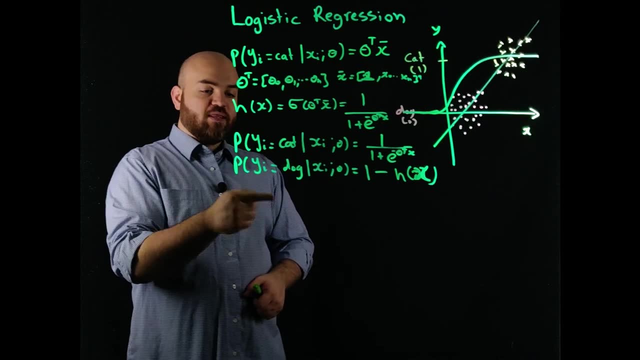 x. I'm confused h with sigma, So h itself is sigma. theta transpose x and that's the probability that I have one class given the input and parameterized by theta, And the other probability is the probability that I'm not of that class or I'm of a different class. I get that And I can. 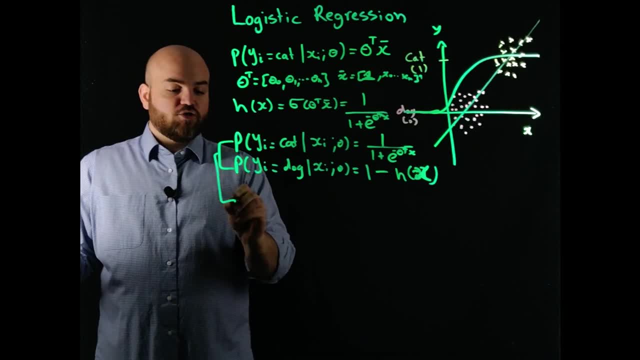 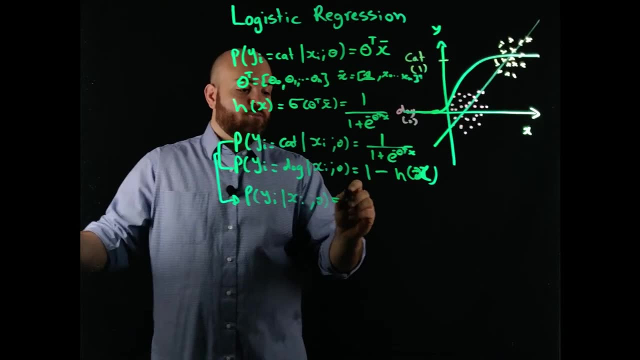 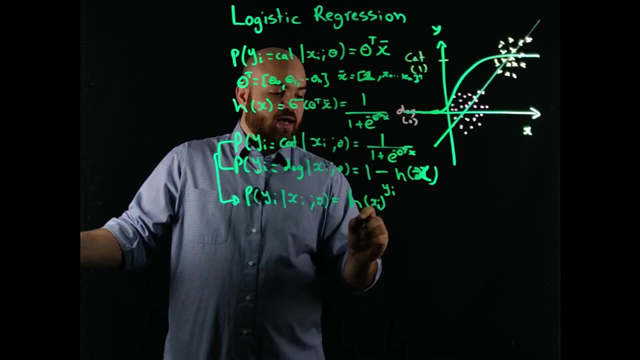 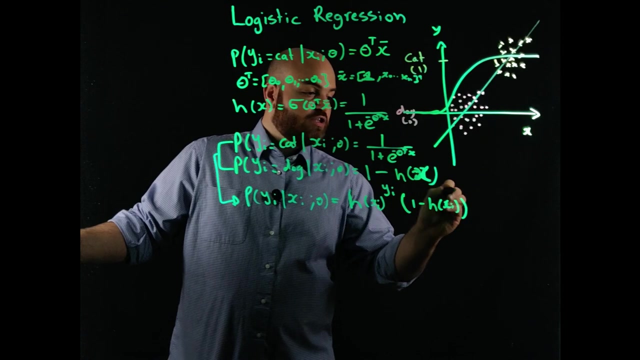 combine those two in one equation and I can say that the probability of yi given xi, parameterized by theta, is equal to the probability itself of hx to the power of yi. so hxi times 1 minus hxi to the power of 1 minus yi. So now this: 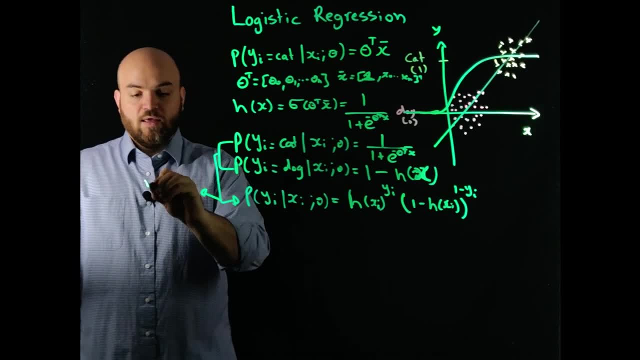 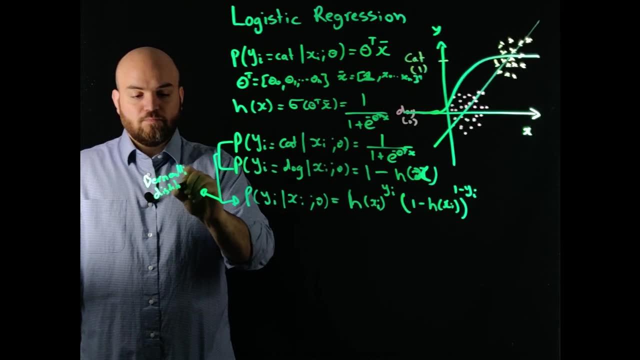 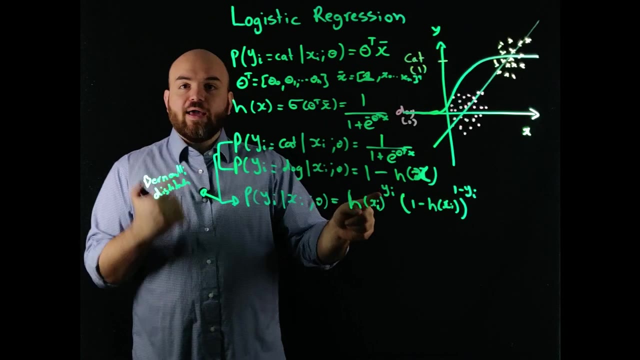 function right here is known as a Bernoulli distribution, And this is nice for a binary problem like this. You see, we have two classes In the case where yi is 1, so my class is a cat, this term remains And this term is 1 minus 0,. 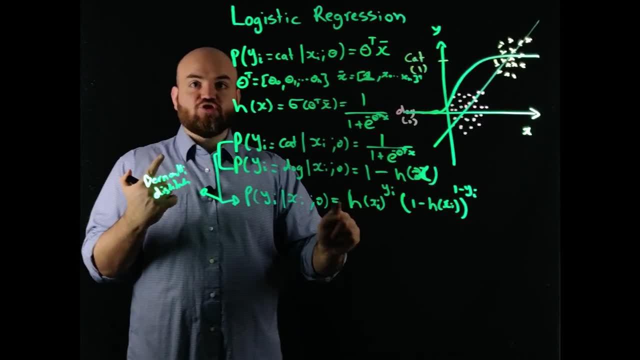 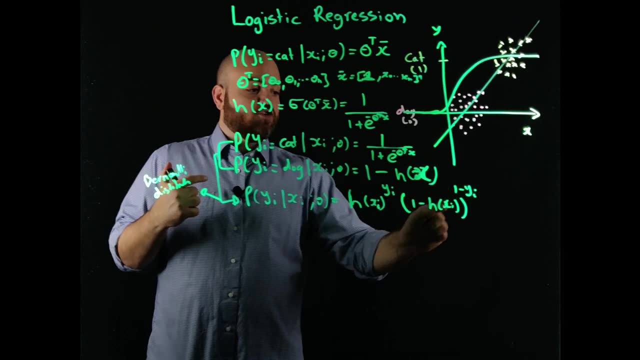 so this becomes 0,, this becomes 1.. So I get hx, so that's the probability that I have a cat. And then if yi was 0, this term becomes 1, and then this term remains and I have the probability. 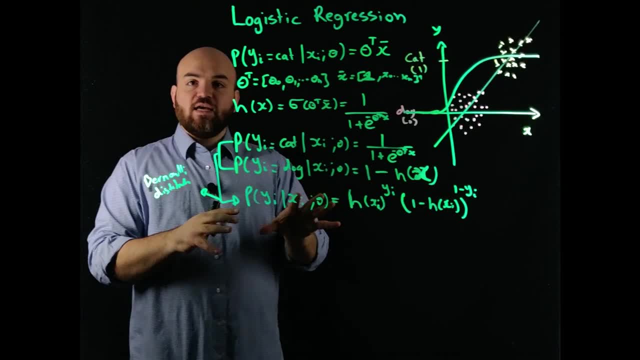 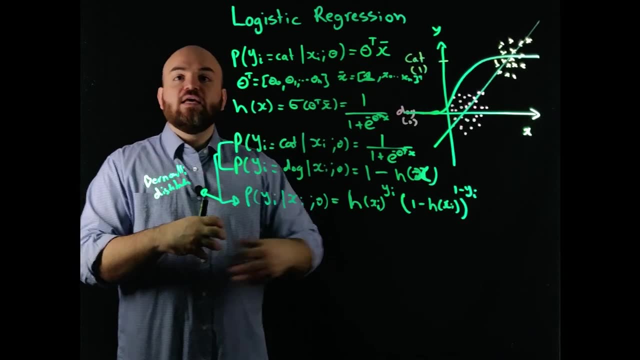 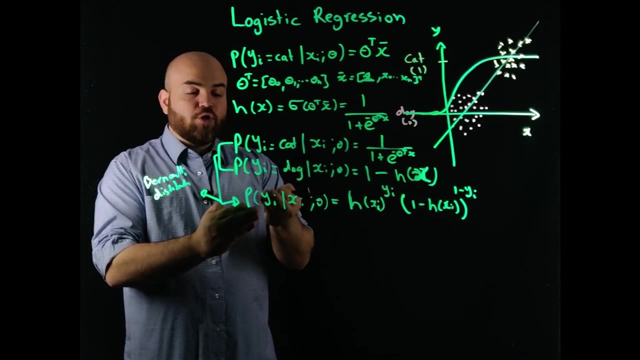 that it's not a cat or a dog. Now, what we're going to discuss here is only for a binary classification problem to show the essence of logistic regression, but it can be expanded to multi-class classification problems. Okay, so now that I have the probability function, this tells me how plausible that my dependent 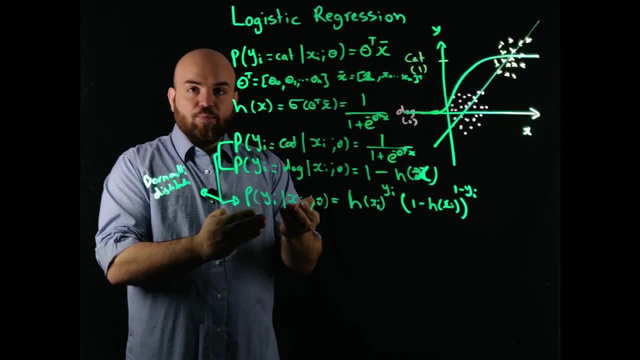 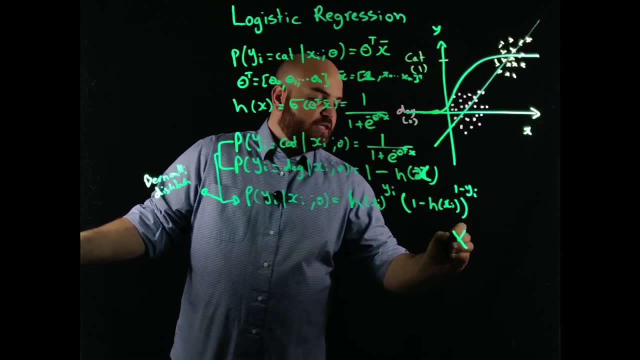 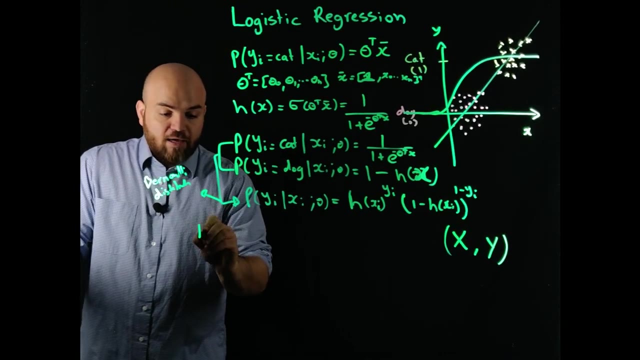 variable is equal to a certain class, given an input with a model parameterized by theta. So if I combine all my observations into a large matrix x and a large matrix, a large vector y, like if I stack them all on top of each other, I can write the probability. 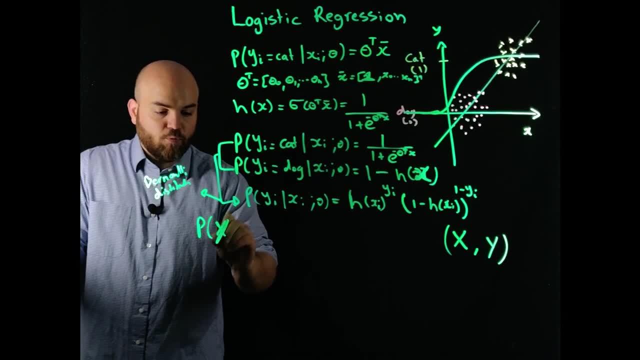 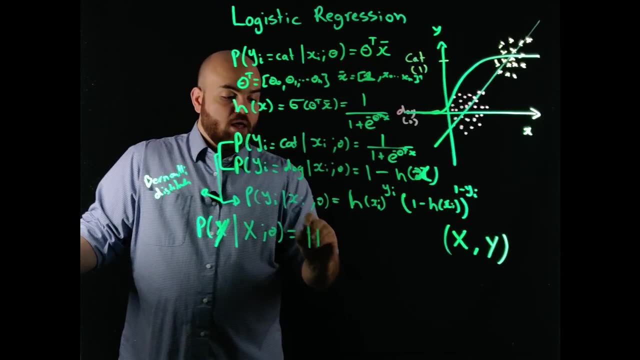 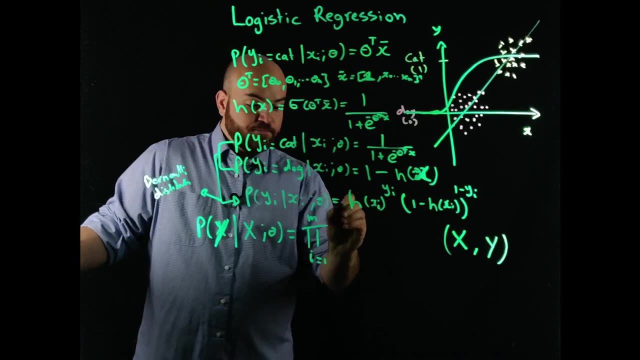 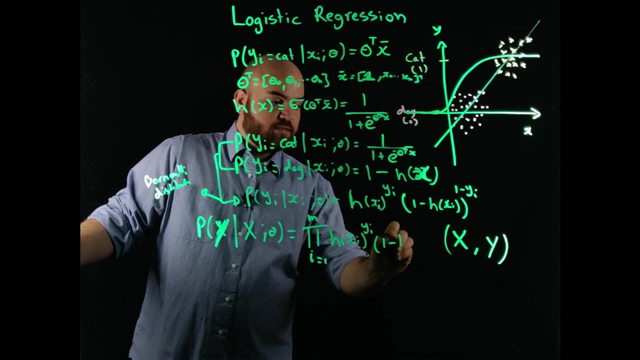 of this is y capital Y, given capital X, parameterized by theta, equal to the multiplication from i equals to m, where m is all of the data points that I have. the number of data points of my hypothesis to the power of i: 1 minus. my hypothesis to the power of 1 minus yi. 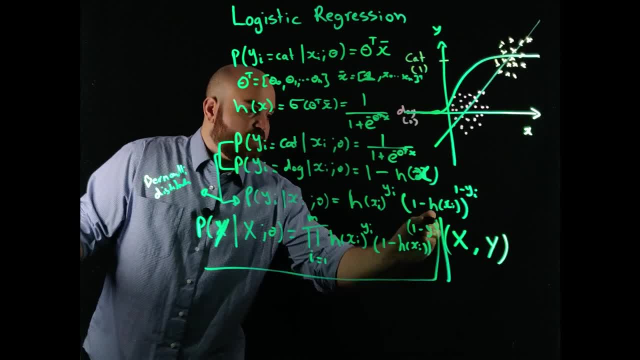 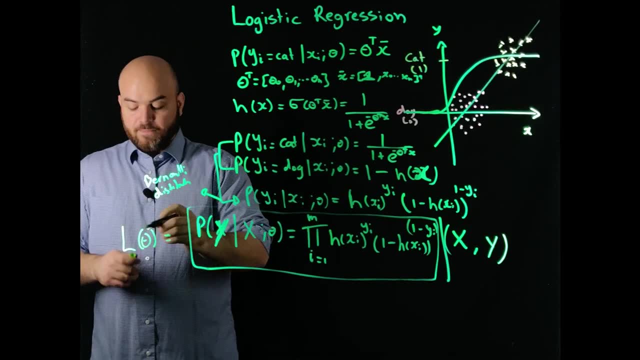 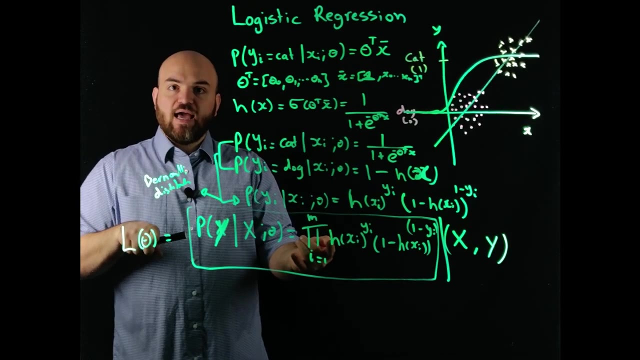 And this whole function right here is typically referred to as my likelihood of theta. So what this represents is how plausible my model is, theta, the parameters that I have given, all of my data points And the reason why I'm able to multiply them all together. 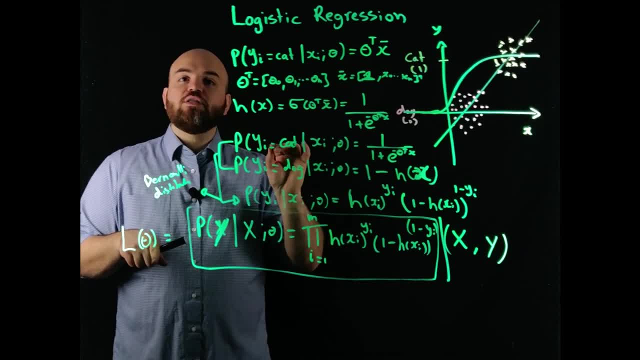 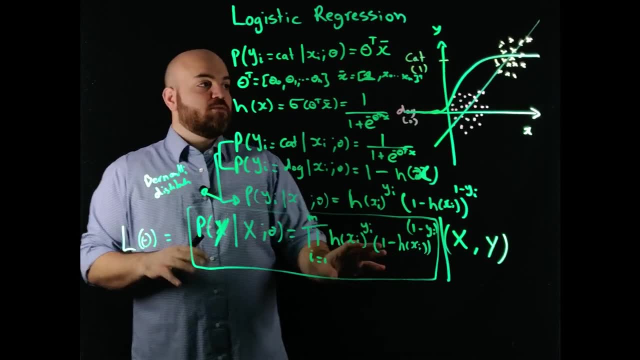 here is because I'm assuming that my data points are independent. So if the data points are independent, I can multiply out all their probabilities and I get the likelihood function. And that is a reasonable assumption, since if I have a picture of a dog or a cat, they're. 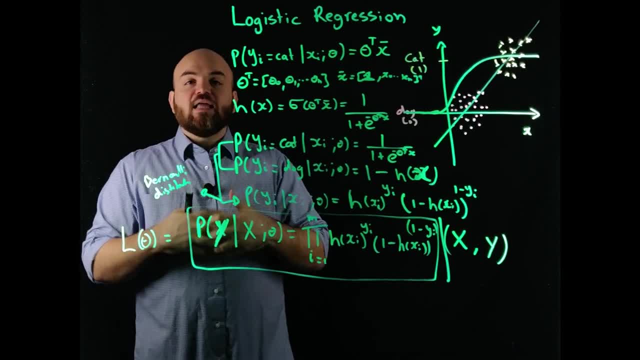 not really related. Even if I have multiple pictures of dogs, they're not dependent. It doesn't matter what camera you took it with. it doesn't matter if you took it with a cell phone, it doesn't matter if it's the same dog. All that matters is that's an image of 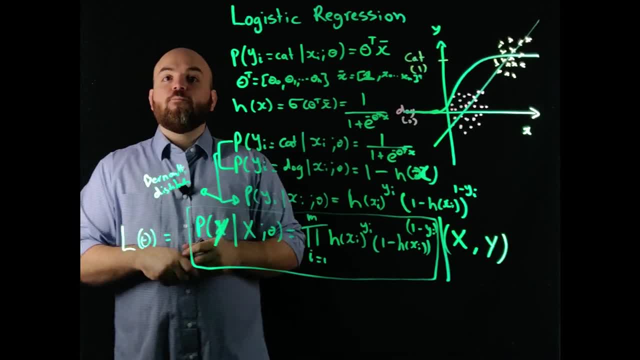 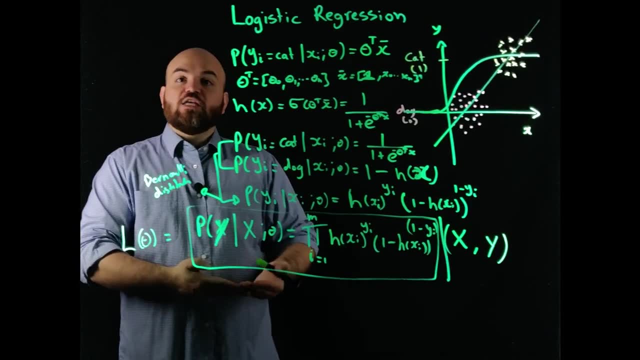 a dog or an image of a cat, and I'm trying to find a model that allows me to predict, given a new image, if that's a cat or a dog. So, this likelihood function, it's what's going to allow us to find these theta parameters. So, now that we have 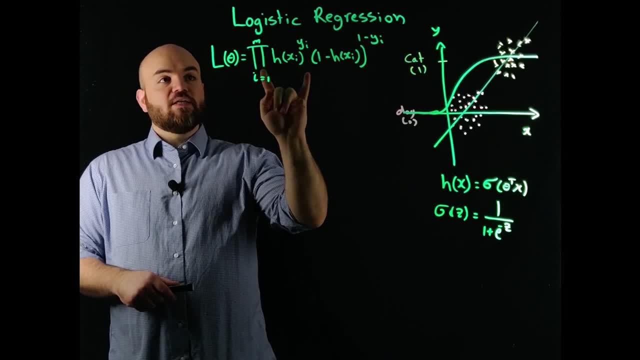 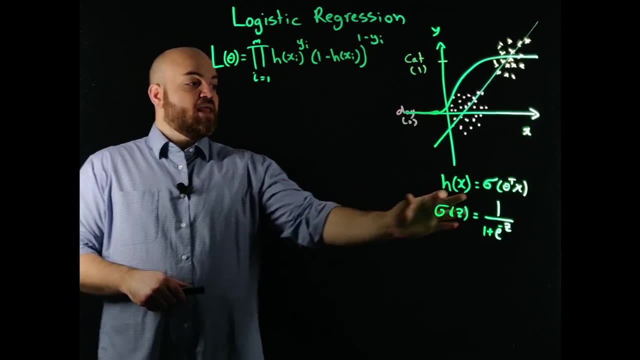 our likelihood function, which represents the plausibility of a model theta parameters. given all the data sets, the data set data points that I have, and I know that my hypothesis uses a sigmoid function- how do I find my model parameters? How do I find the thetas? 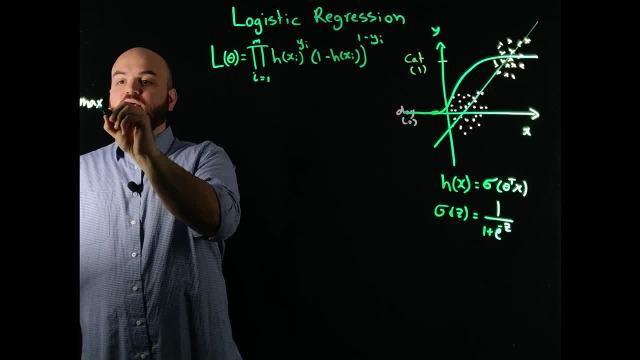 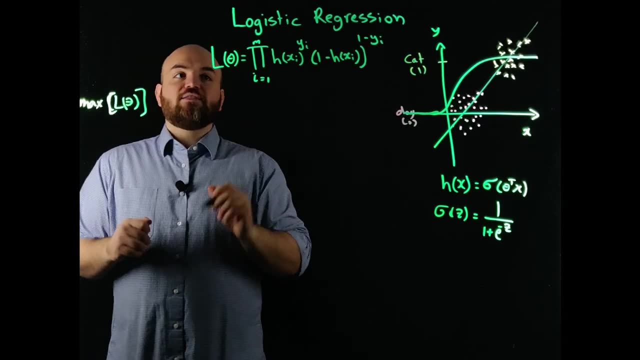 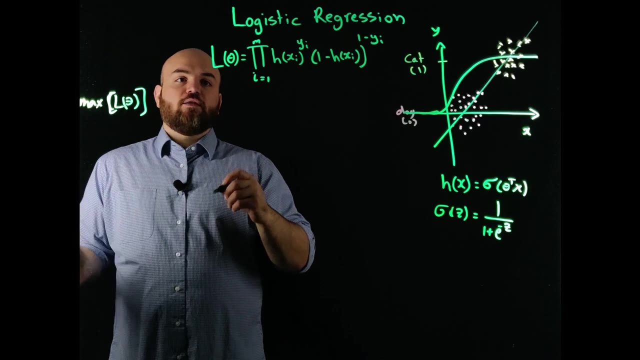 Well, the way to do that is to maximize my likelihood function right, Lof, theta and theta. and that's not easy to do when i have multiplication of probabilities. so one way to deal with this is to use the log likelihood. so if i take the log of this likelihood function, 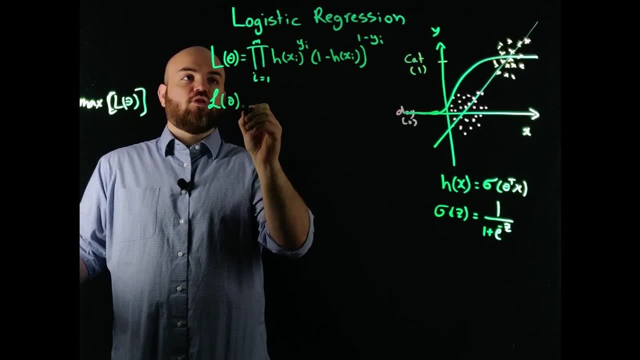 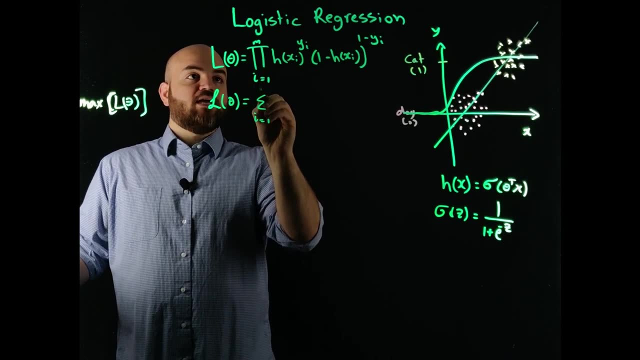 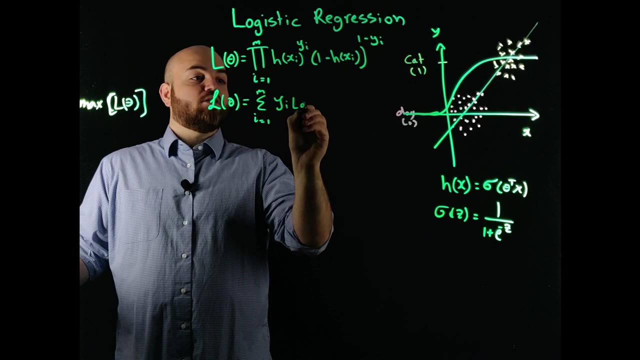 i'm going to write it as you know, script l of theta. so the log likelihood. if i take the log, the nice thing is this: multiplication becomes a sum and that's a nice property of the log. and then i have this exponent becomes a multiplier times the log of the hypothesis, which is sigma. 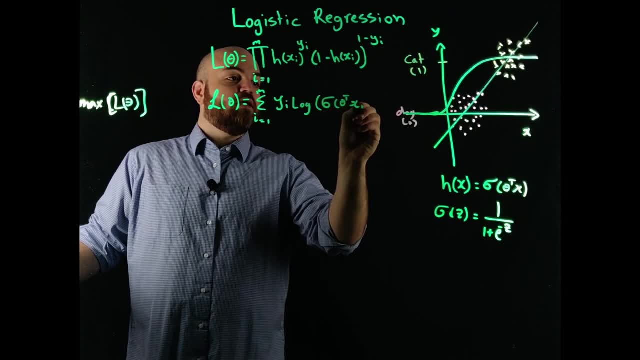 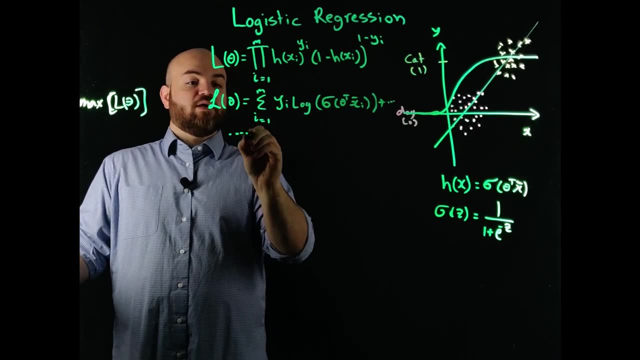 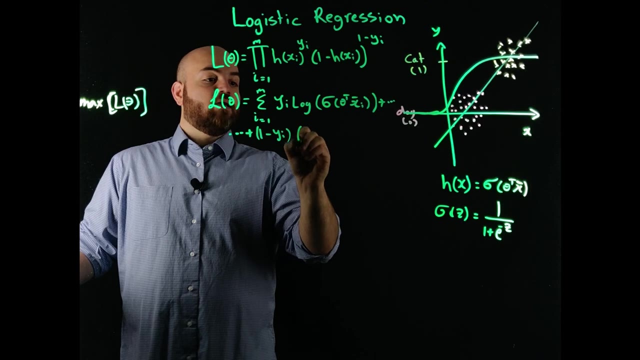 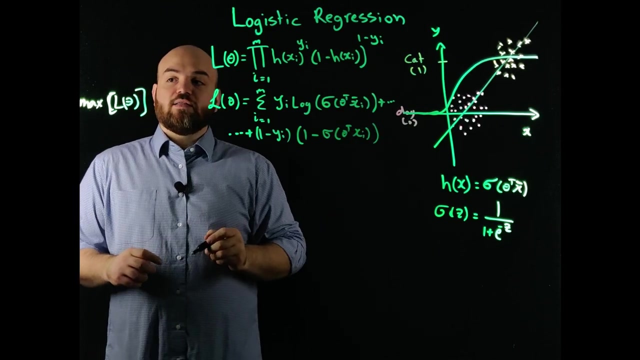 sigma of theta transpose xi bar. this is bar right, and then i have plus, because the multiplication becomes a sum, this exponent becomes a multiplier and multiplied by one minus sigma of theta transpose goes xi. So this is my log likelihood, So I need to maximize in this case my log likelihood And 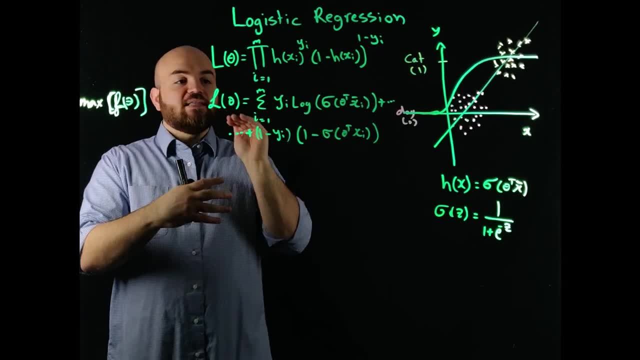 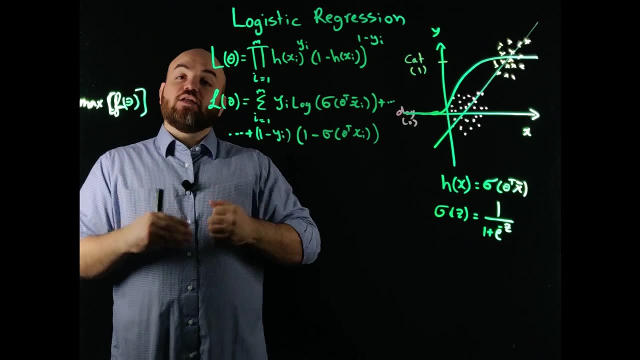 this is nice because to maximize a function I can take the derivative and move in the direction of the gradient, So I can do gradient ascent. In our last video in linear regression we talked about gradient descent because we wanted to minimize a function. In this case we want to. 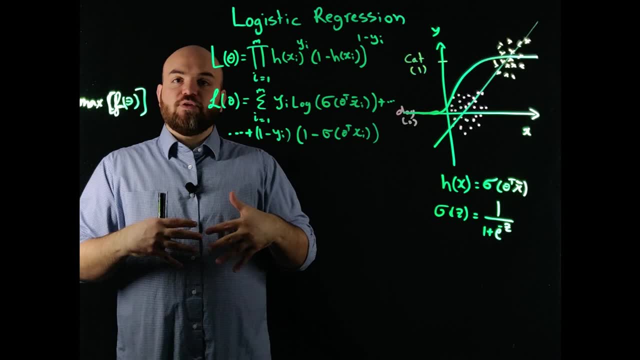 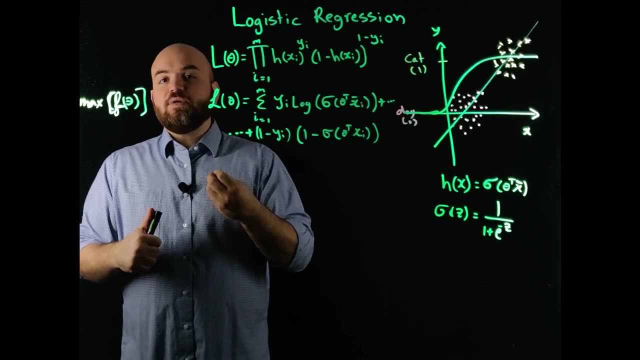 maximize the likelihood or the log likelihood. The reason for that is, since the likelihood represents the plausibility of my model, if I maximize it intuitively, that means that that's the most plausible model that I can use to represent this data. Okay, so let's go ahead and do that. 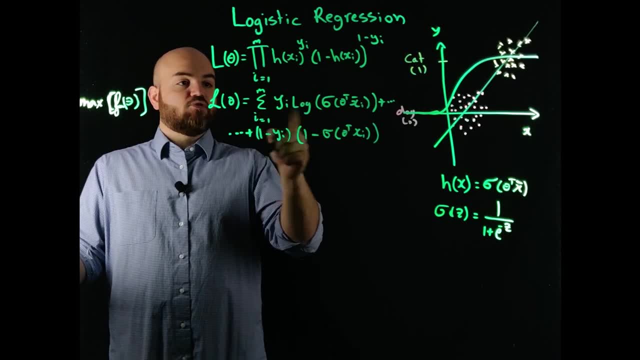 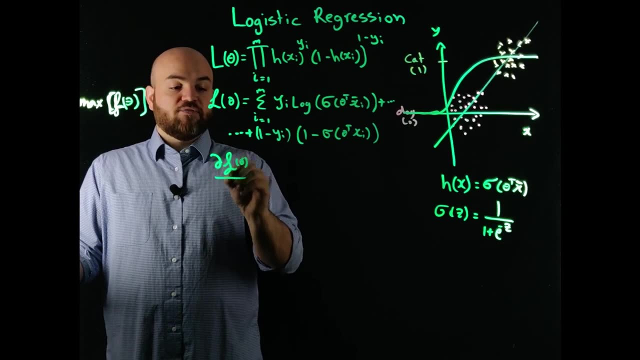 So if we looked at one data point, so I'm going to drop the i subscripts and the sum because they're not affected by the derivative- And if I'm going to take the partial derivative of this log likelihood as a function of theta with respect to theta, what do I get? My y derivative of that is: 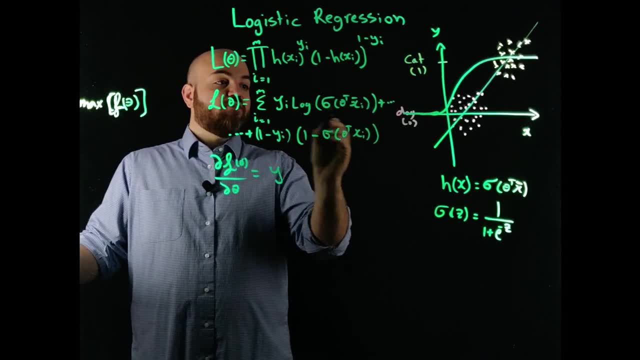 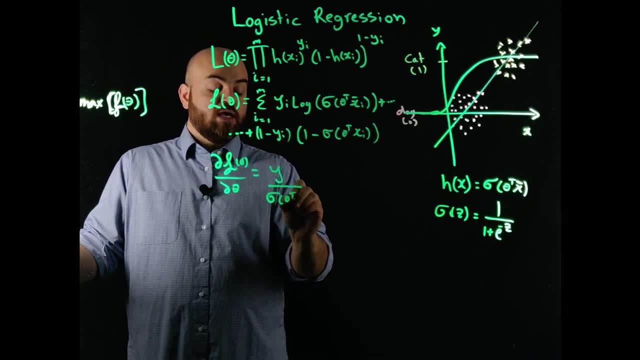 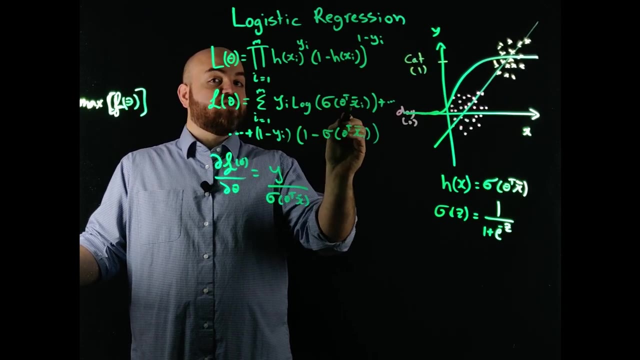 zero. so I don't care about that, so I keep going. And then the derivative of a log is one over whatever is inside the log. and let's say sigma of theta transpose x, bar, And then I have the derivative of this term whatever is inside the. 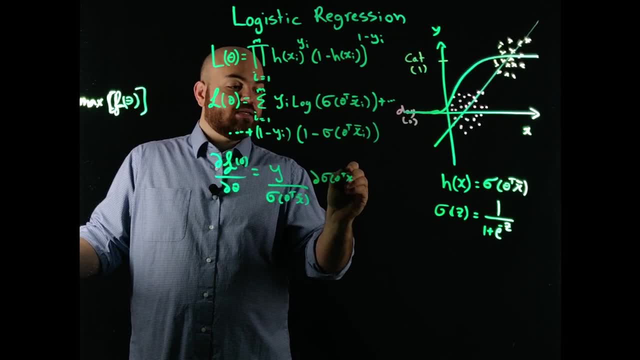 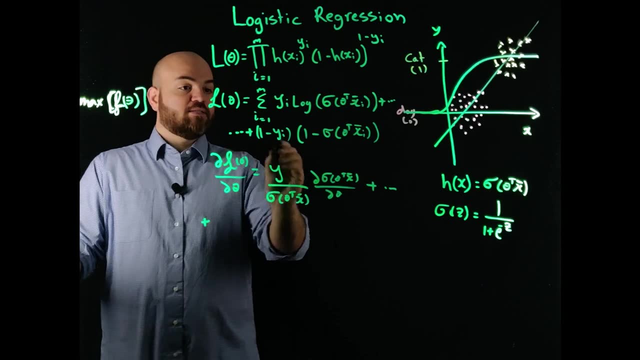 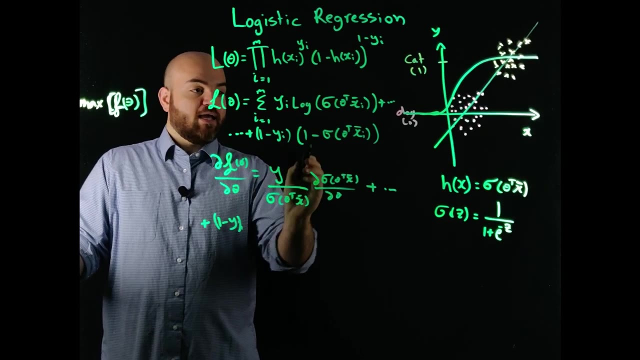 log. So the derivative of sigma theta transpose x bar divided by derivative of theta, And then I have plus. The other term is going to be one minus y. can't take the derivative of that. there's no theta in there. drop the i And then I have. 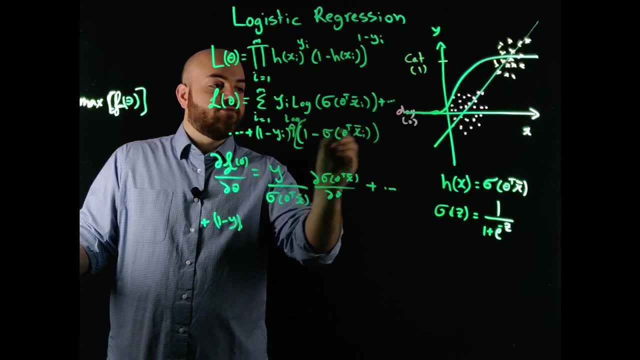 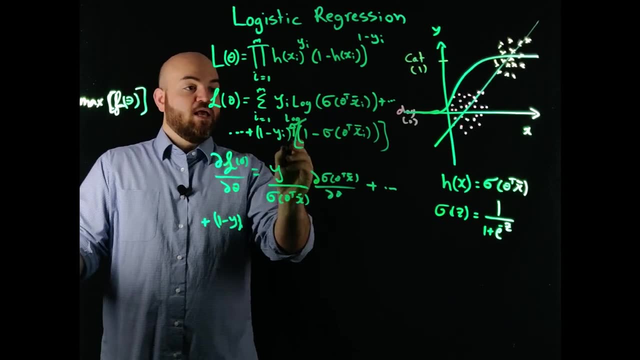 oh, there is a log here. I'm sorry, this is log of this value, right, Because there's a log here. there should be a log here, because I have a log expanded in all this whole function. So the derivative of a log is one over whatever is inside that log, which is, in this case, one. 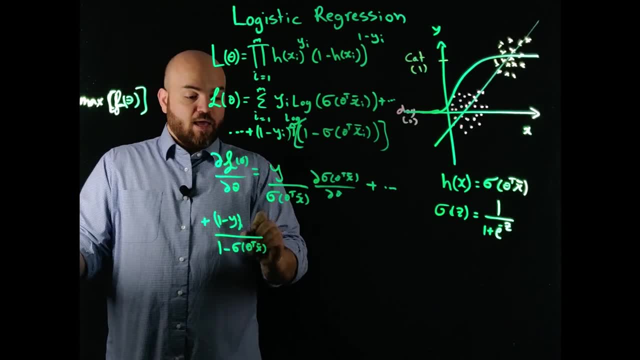 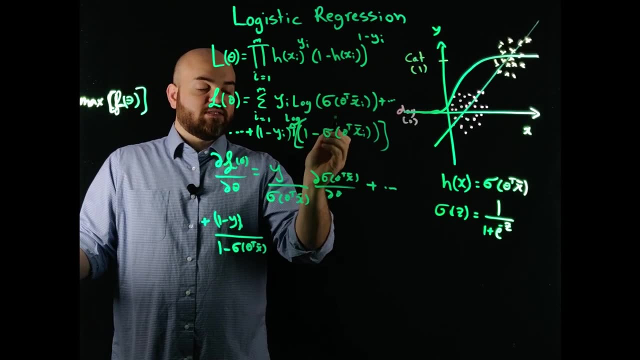 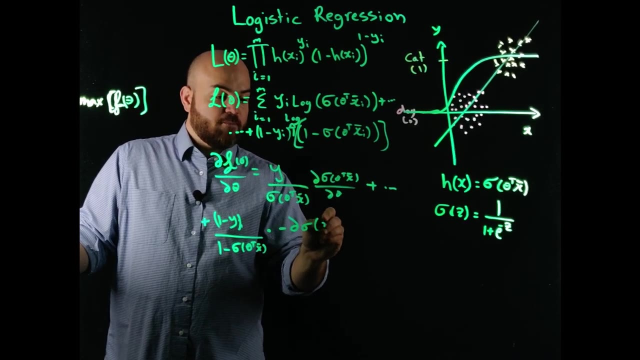 minus. sigma of theta, transpose x, bar. And then I multiply with the derivative of this term with respect to this, So this one derivative is zero, goes away. so I have a negative sign. so dot product. negative sign of this derivative. so the partial of sigma theta, transpose x, bar. 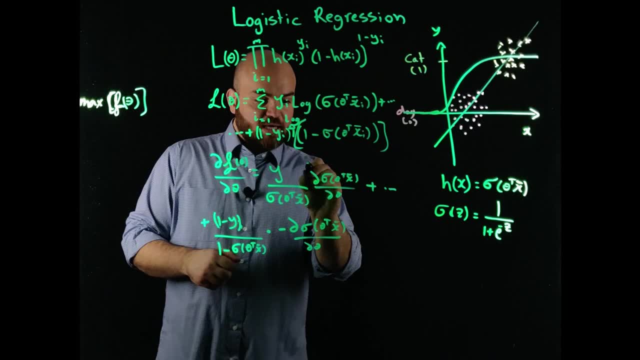 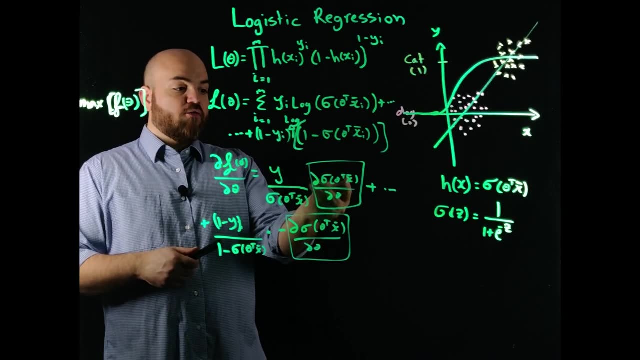 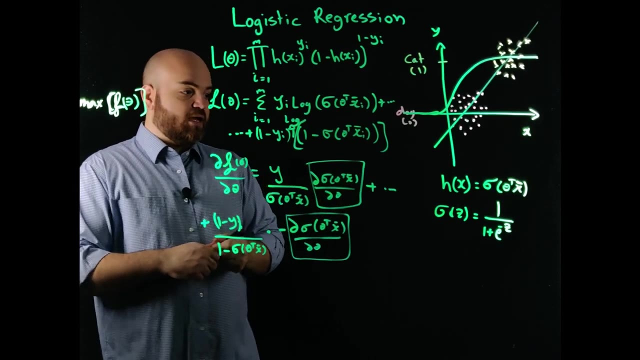 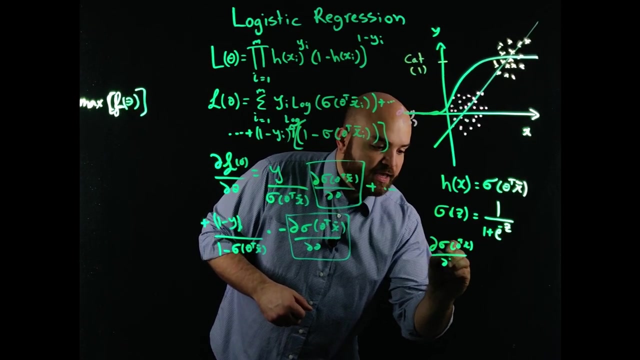 with respect to theta. So you can see, here I have this term and this term shared And this is essentially the derivative of the sigmoid with respect to theta. So the sigmoid has a theta transpose times x, right? So I can write the derivative of sigma: theta transpose of x by theta. 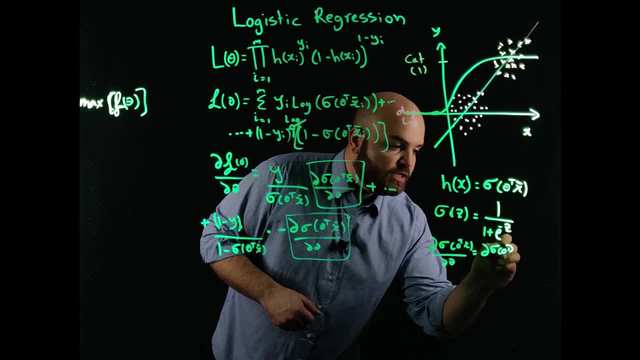 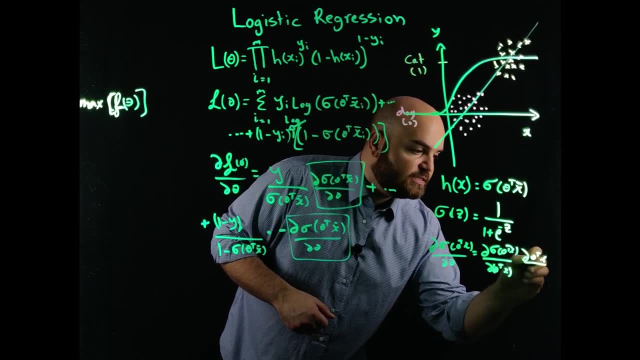 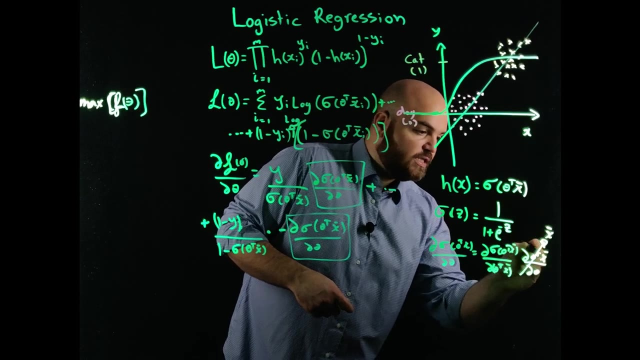 as the derivative of sigma theta transpose x by the derivative of theta transpose x multiplied by the derivative of theta transpose x divided by the derivative of theta. In this case, this value is basically sorry. these are all x bars. This value is x bar. 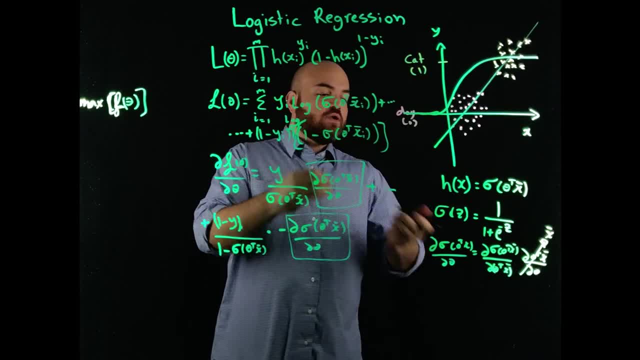 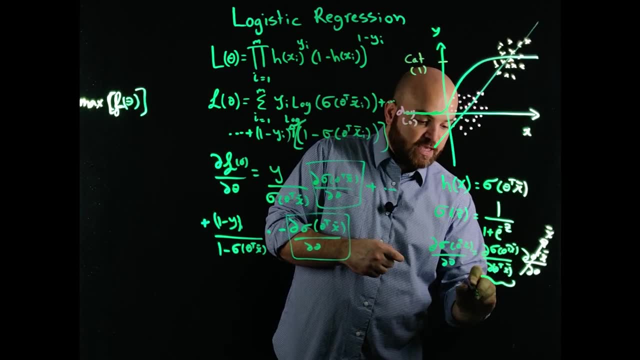 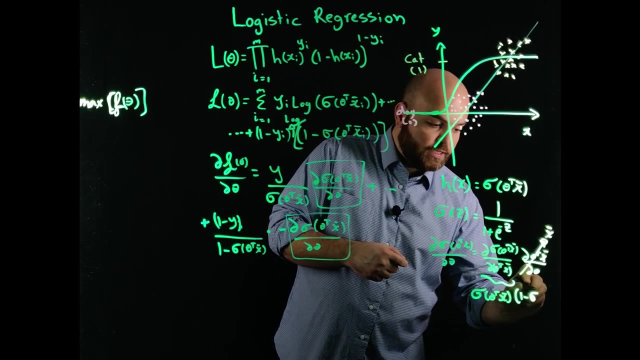 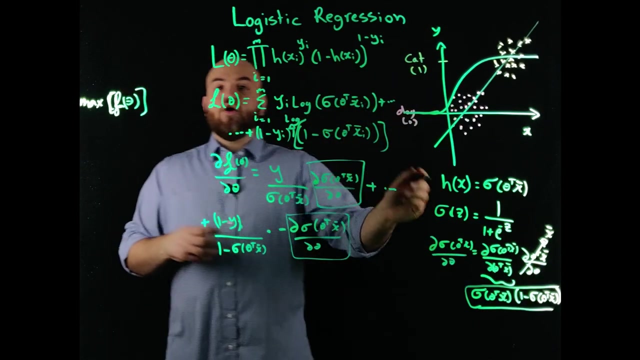 and this value is the derivative of a sigma. And this is where the mathematical convenience of a sigmoid comes into play, because the derivative of a sigmoid function with respect to its input is essentially the sigmoid itself multiplied by one minus the sigmoid itself, And that's very mathematically convenient. So you can go and you can prove that to yourself. 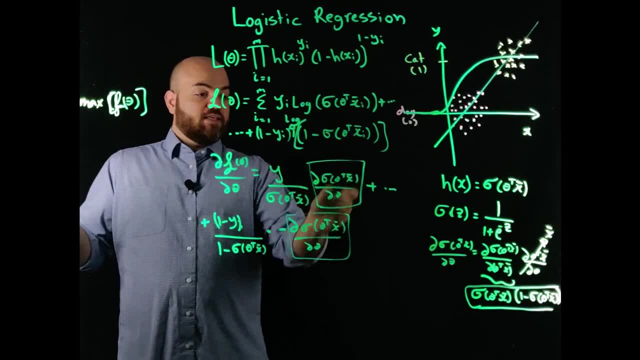 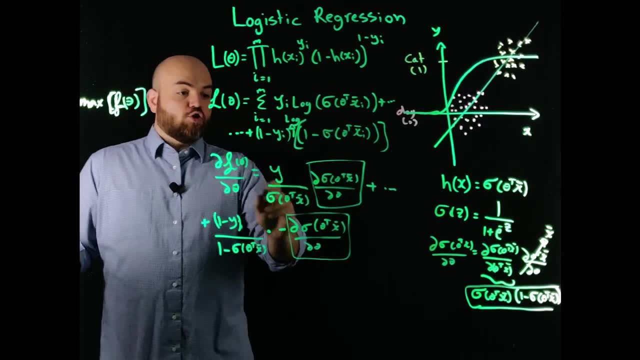 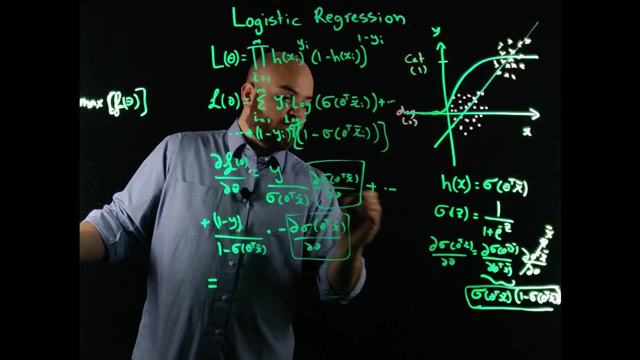 but this is the actual derivative of the sigmoid. So in this case here I know that this term is that and then this term is x, bar, and this is shared with each other. So if you multiply out, you essentially can get. you can show that if I substitute this derivative. 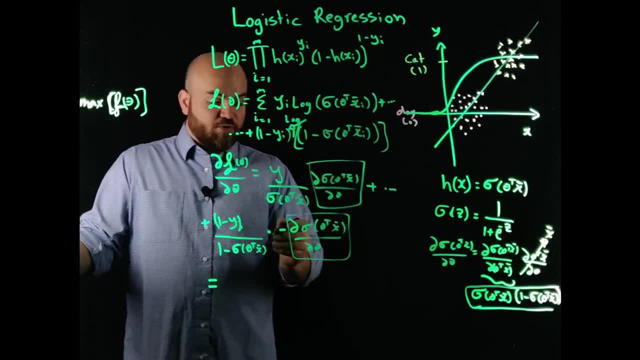 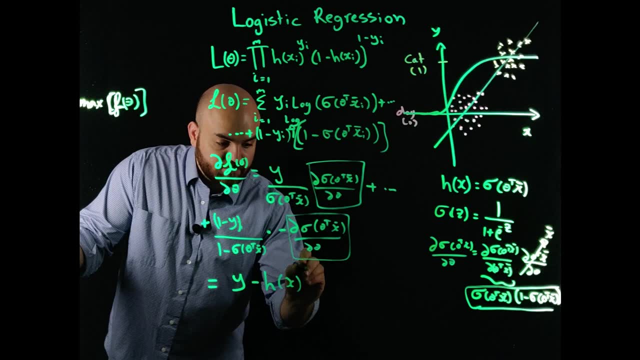 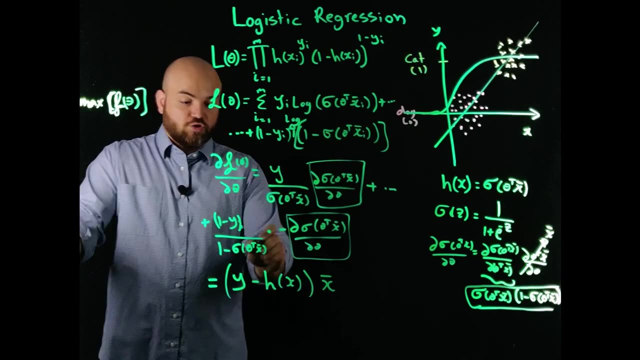 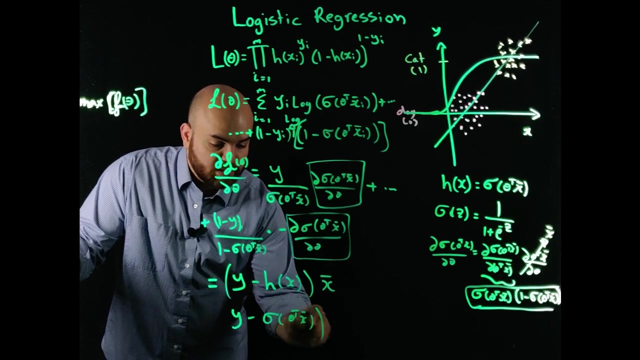 here: times x bar. same thing here, and I multiply everything out. then you can get y minus h of x multiplied by x bar. right, This is what you get. So y itself minus sigma of theta transpose x bar: times x bar. 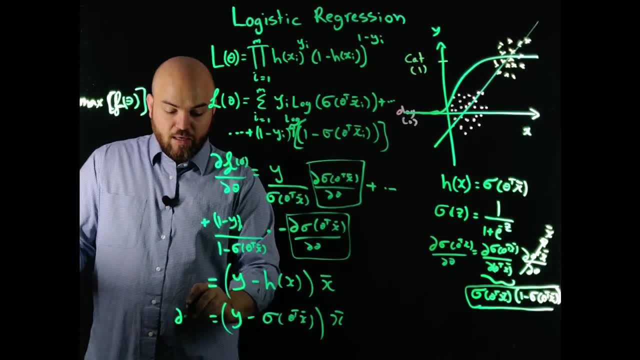 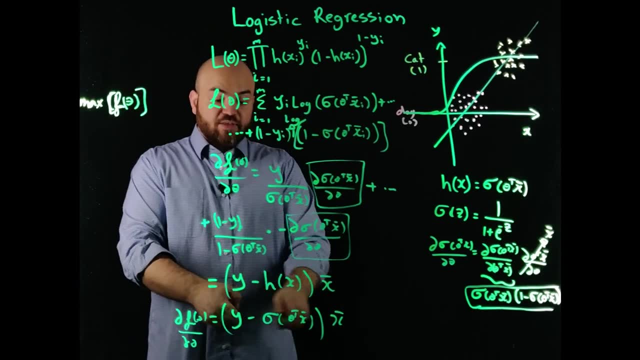 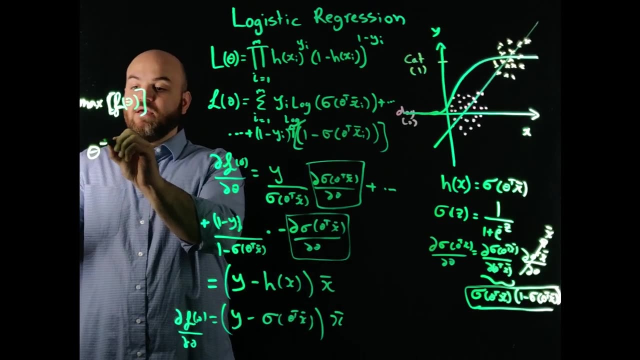 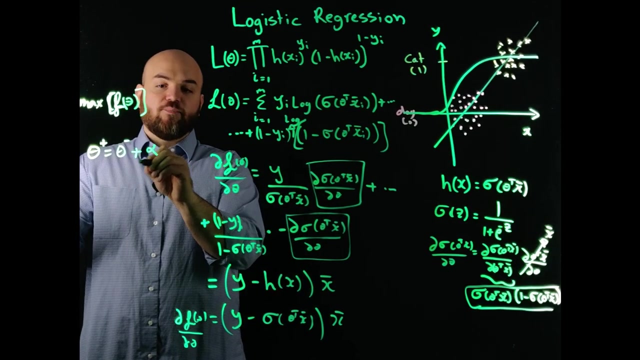 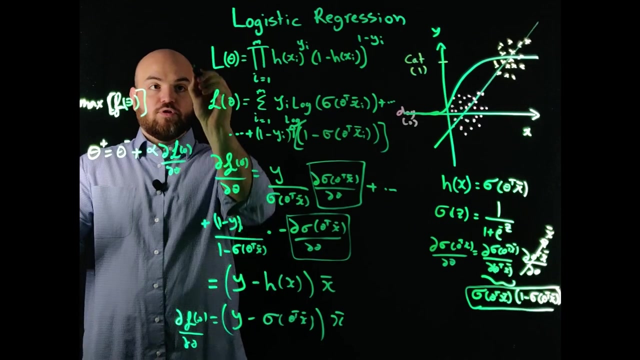 So this is my derivative of the log likelihood of theta with respect to theta And this equation is what I would use for gradient descent to compute my values iteratively of theta until I converge. But this is again gradient ascent, so I have a positive value. alpha times: partial log likelihood with respect to theta. 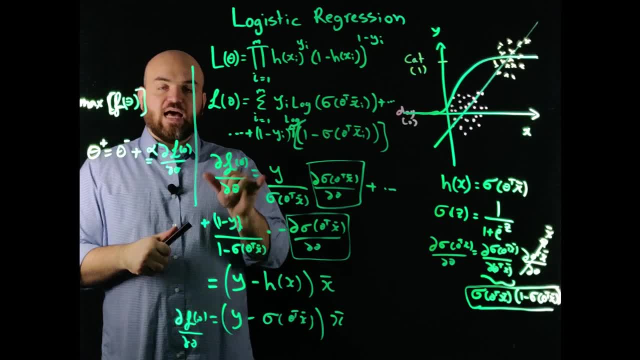 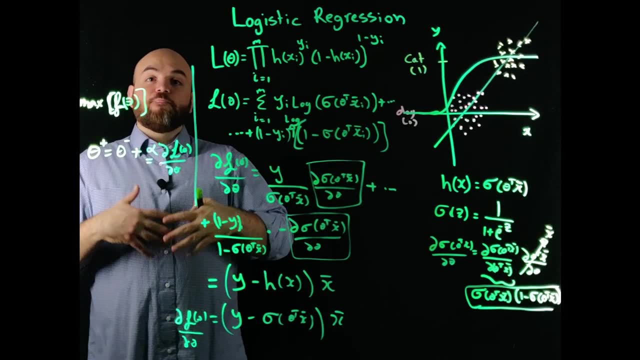 And this alpha is our scaling parameter, our step size, and this is the derivative itself. So there you have it. This is the maximum log likelihood approach to finding the parameter model of the sigmoid function. And this is the maximum log likelihood approach to finding the parameter model of the sigmoid function.